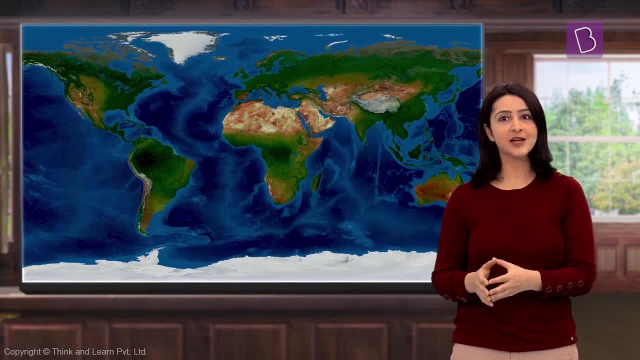 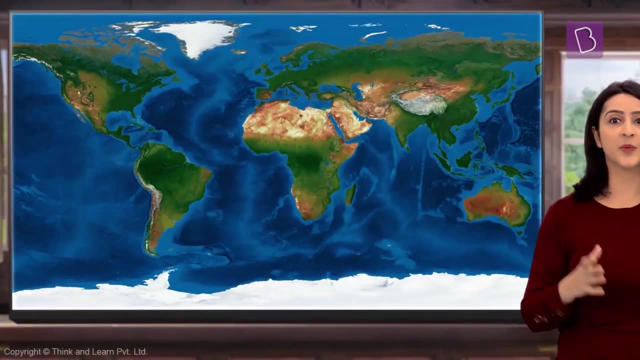 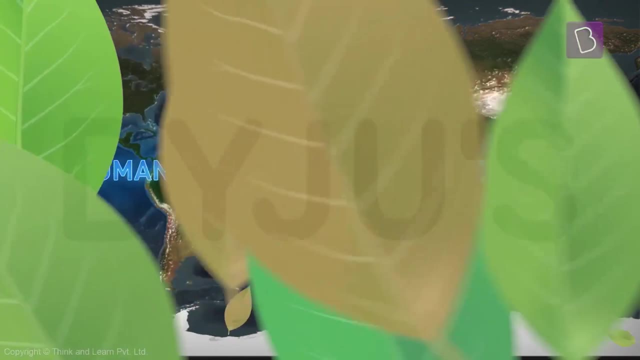 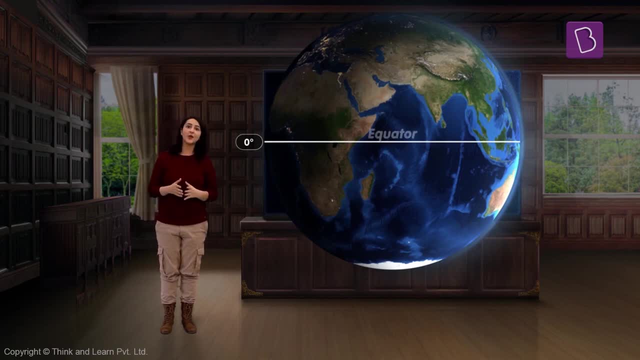 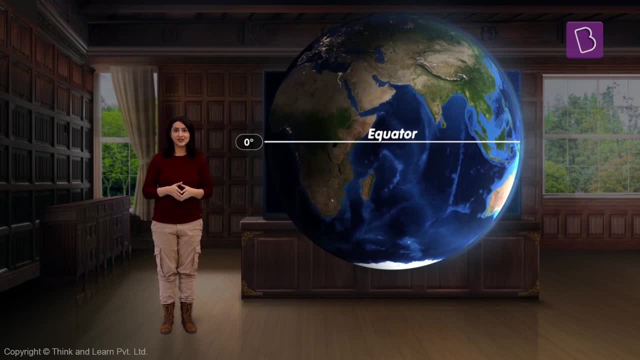 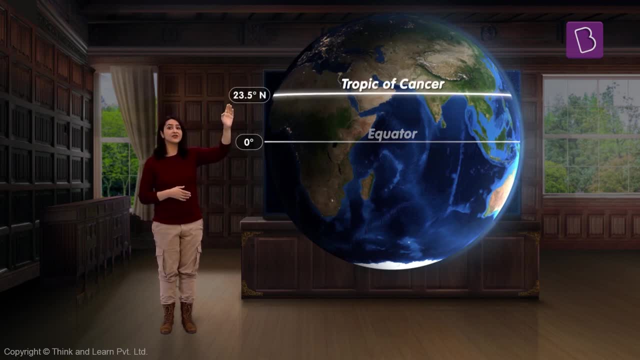 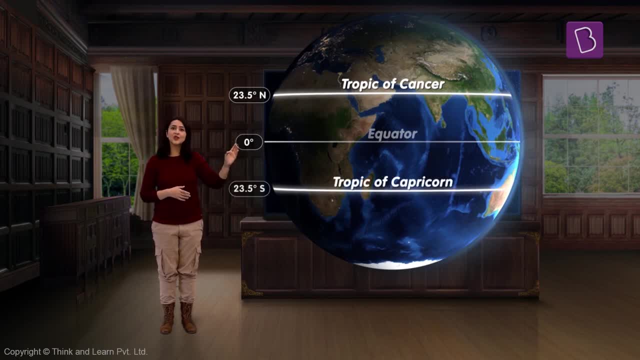 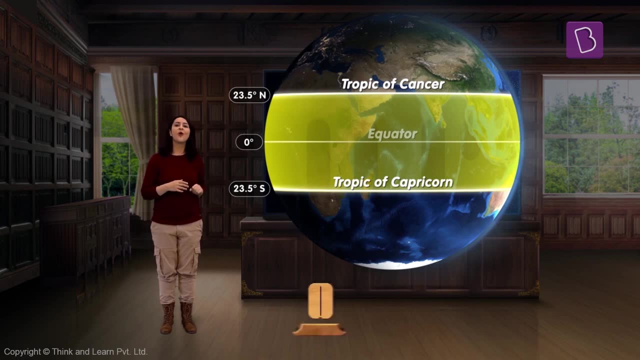 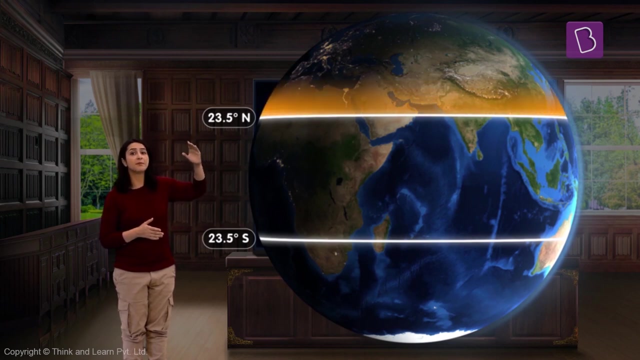 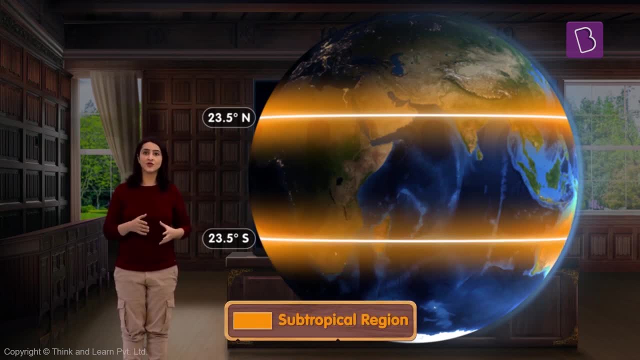 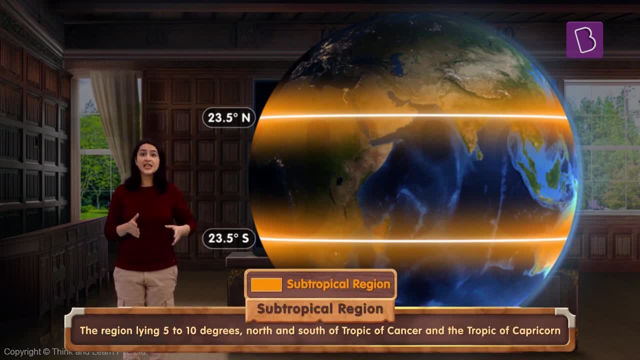 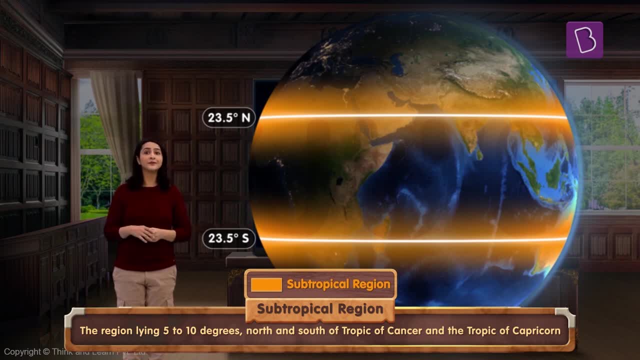 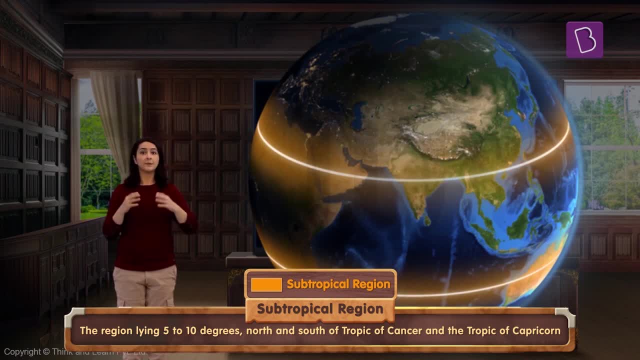 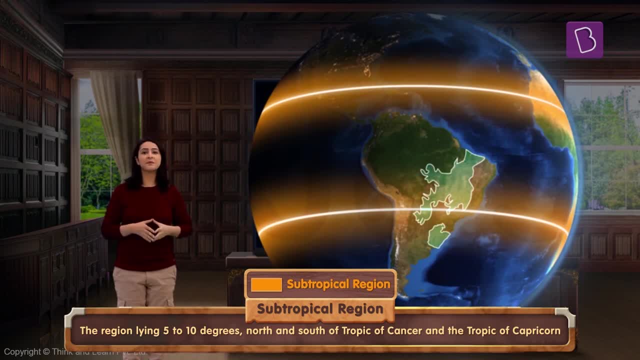 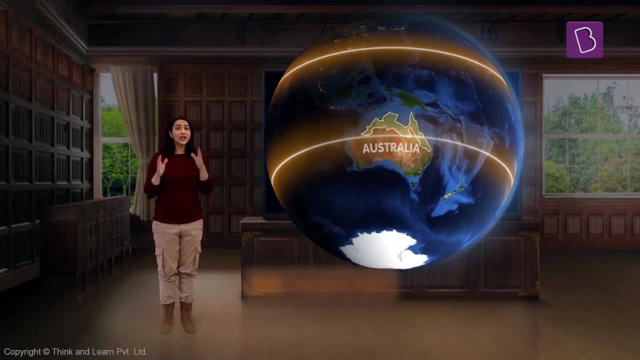 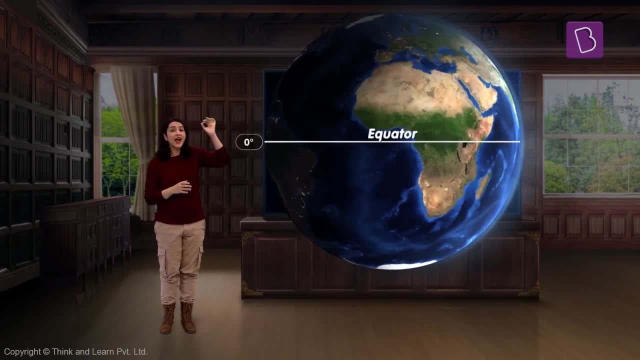 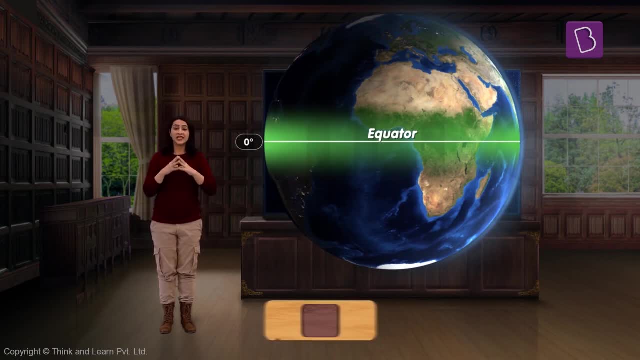 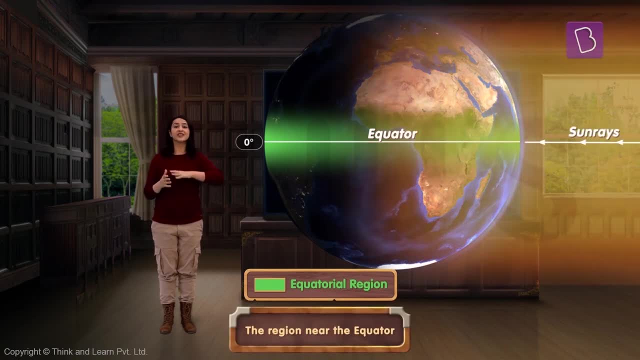 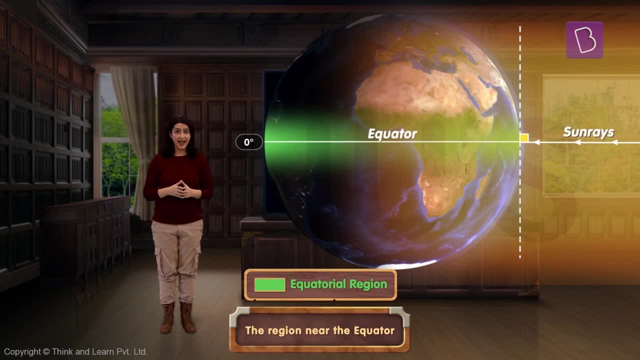 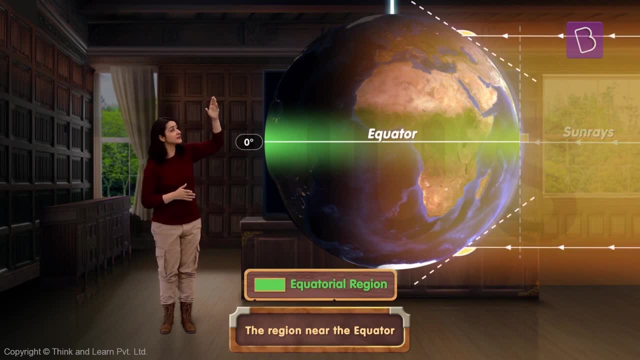 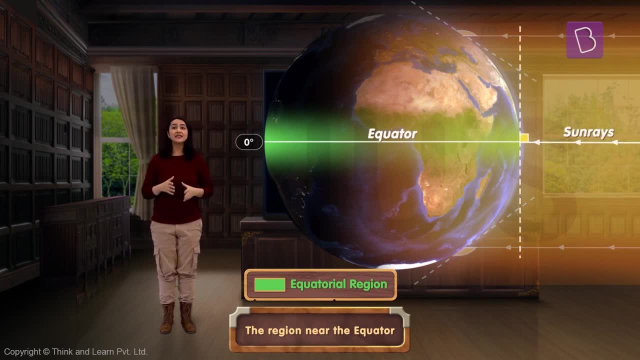 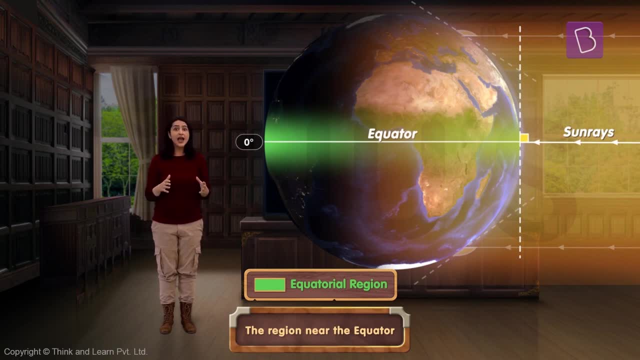 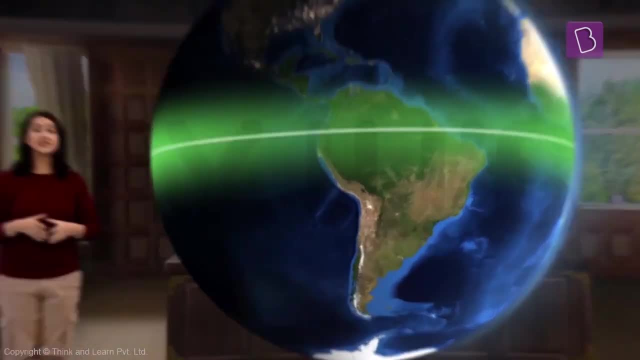 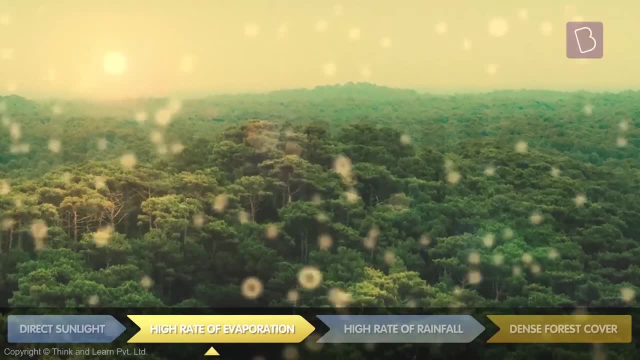 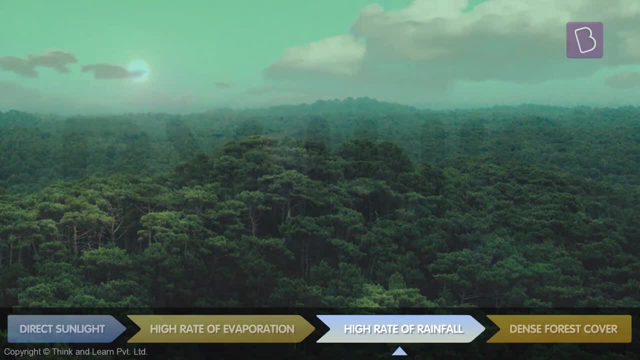 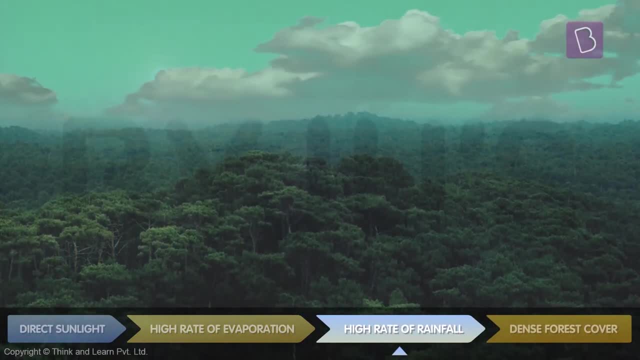 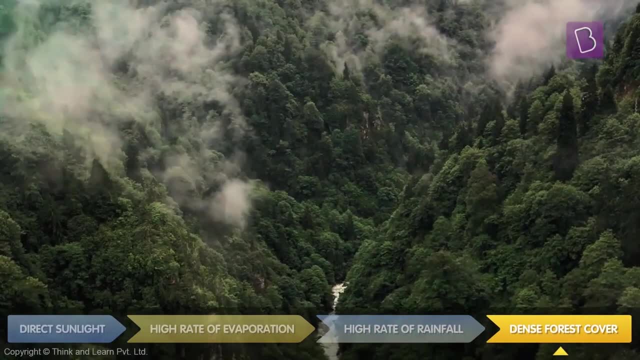 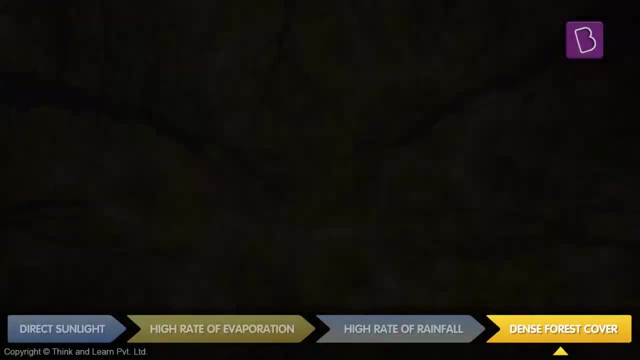 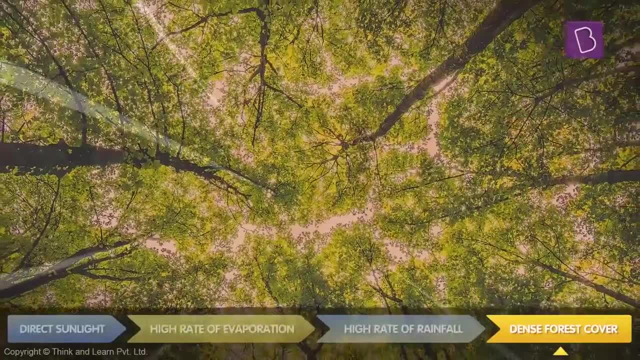 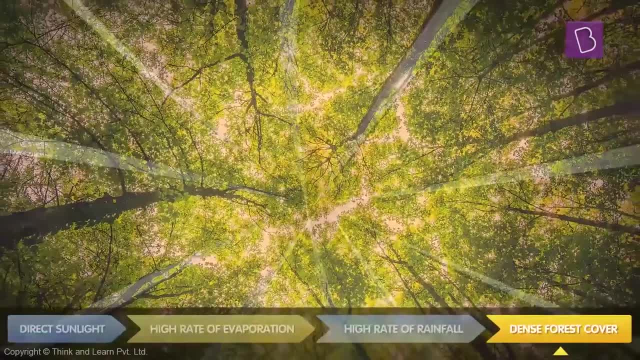 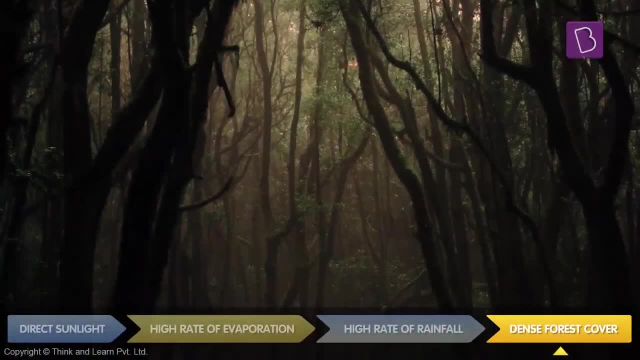 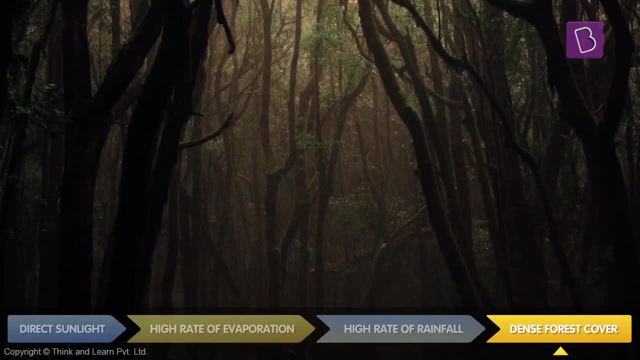 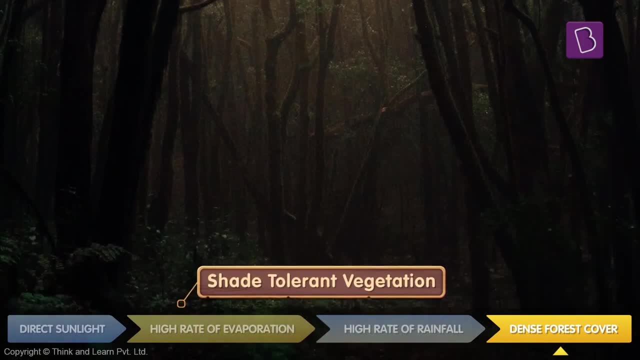 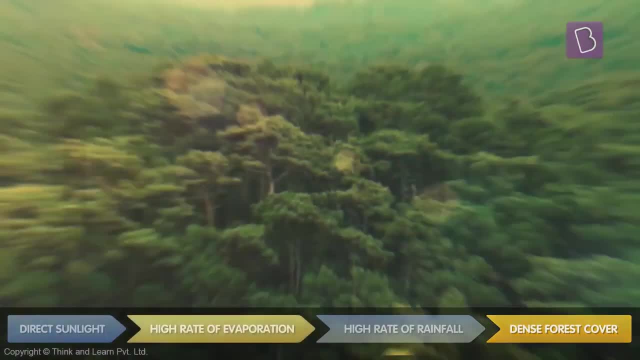 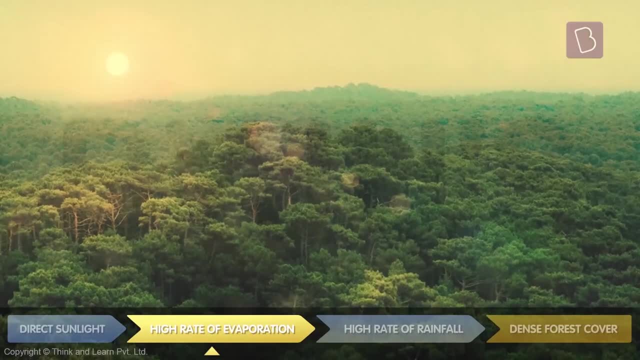 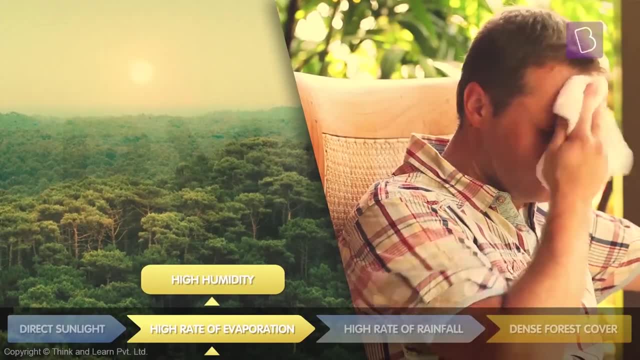 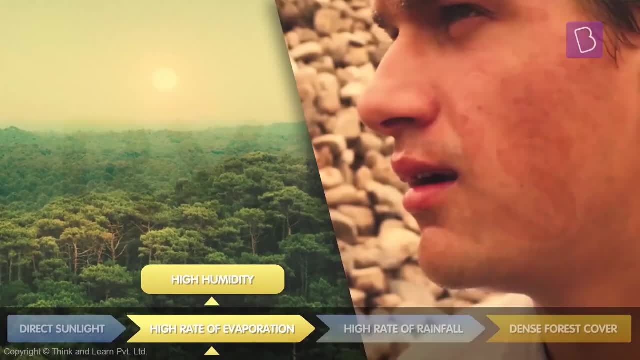 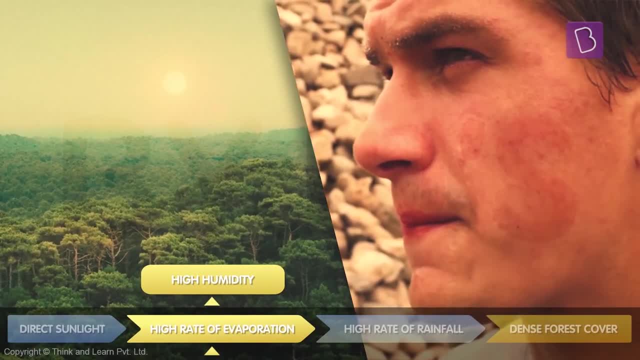 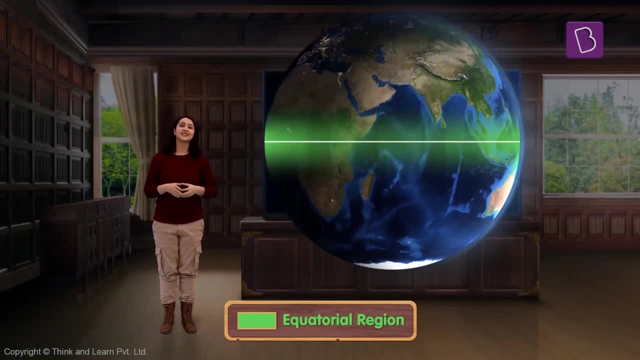 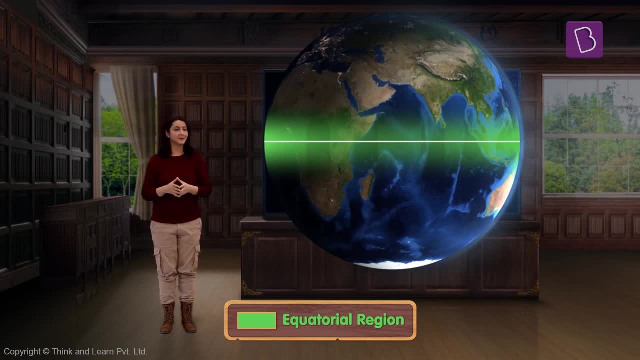 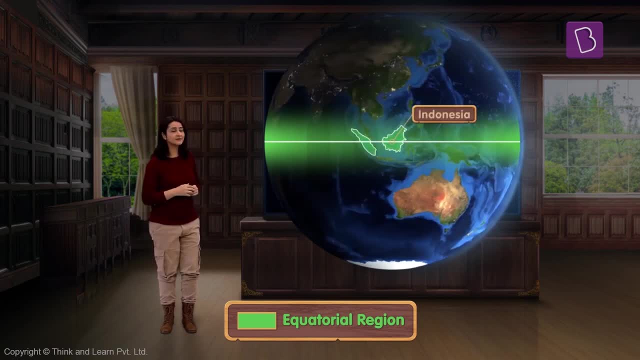 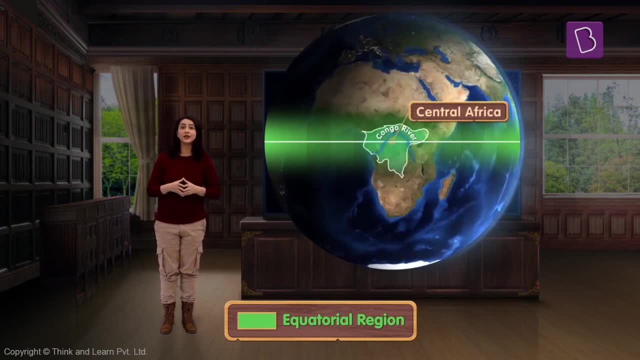 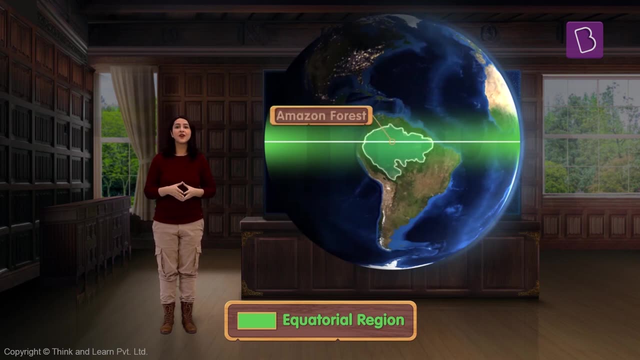 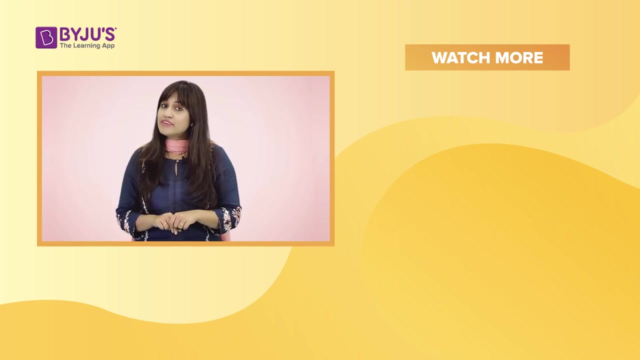 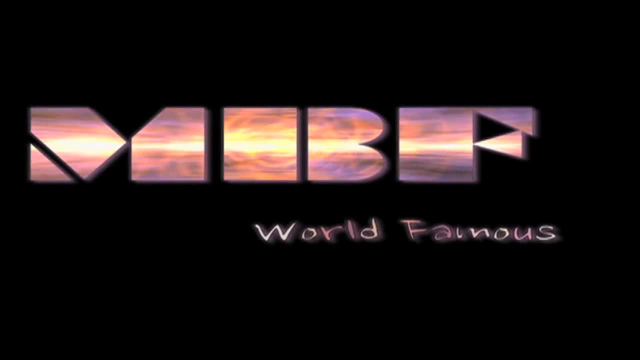 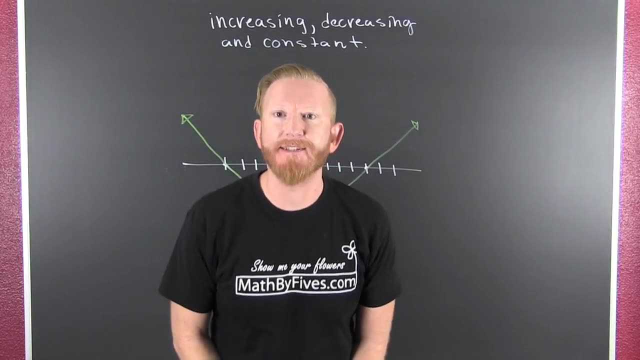 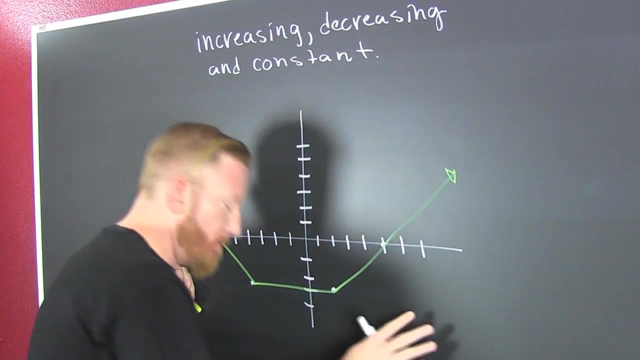 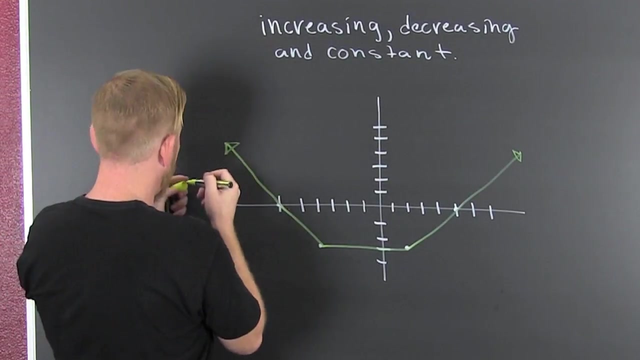 Increasing, decreasing and constant. What From a graph? Aye, Look at this guy. And Who wished that upon me? Anyway, here if we go and we see if We're on a tech deck, Whoa. 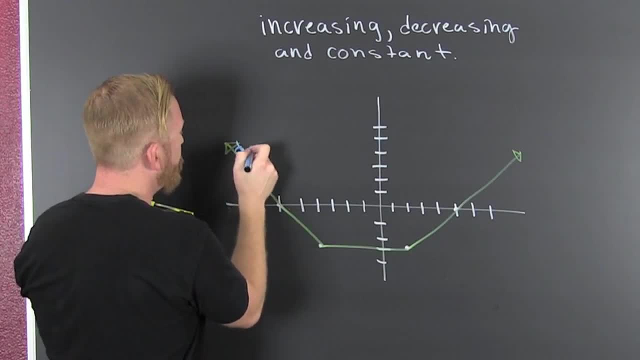 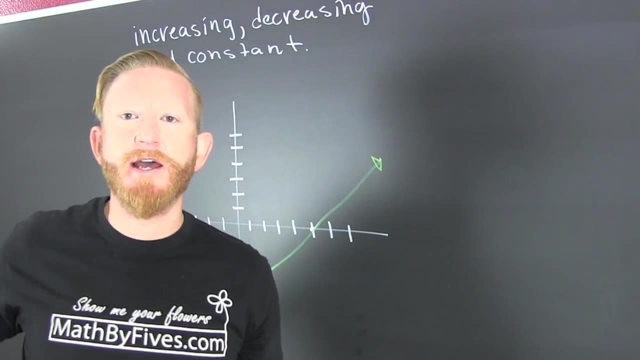 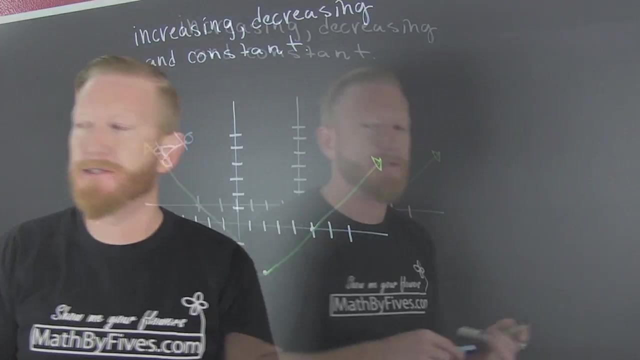 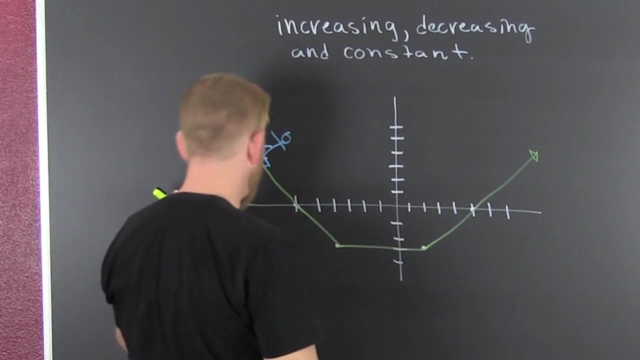 You remember those? That's you, And you're going from left to right, Daniel-san, Left to right. We're always going in increasing order, at X, when we're looking for increasing, decreasing and constant. So if you're on that tech deck and you're all, What do they?